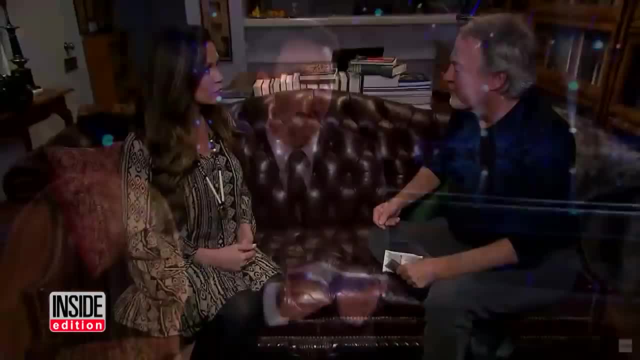 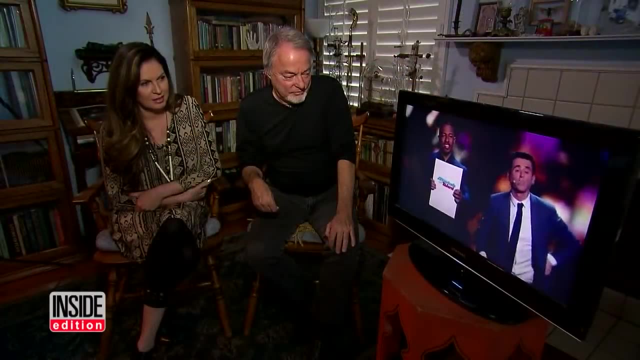 but they wouldn't spill the beans on Perlman's method. So, with the help of author and mentalist Mark Edward, I analyzed this clip. It's a clip from America's Got Talent in which Perlman asked the judges to predict how many gumballs are in a jar. 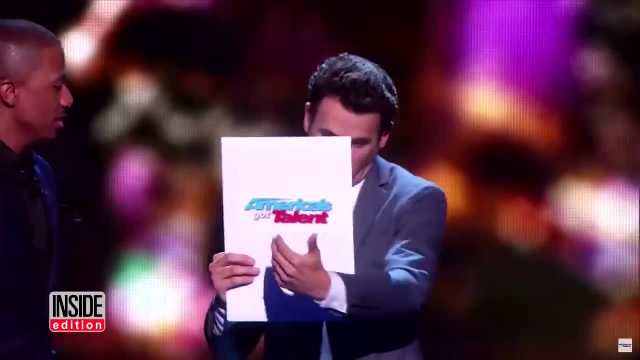 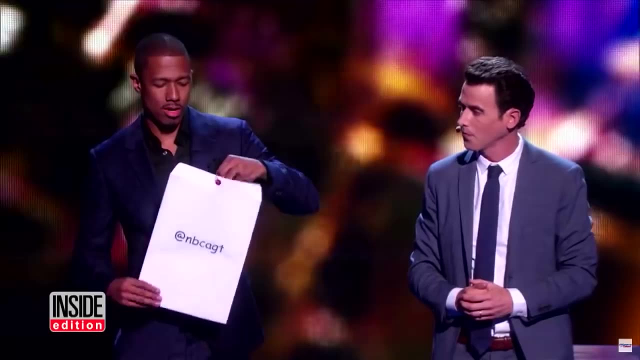 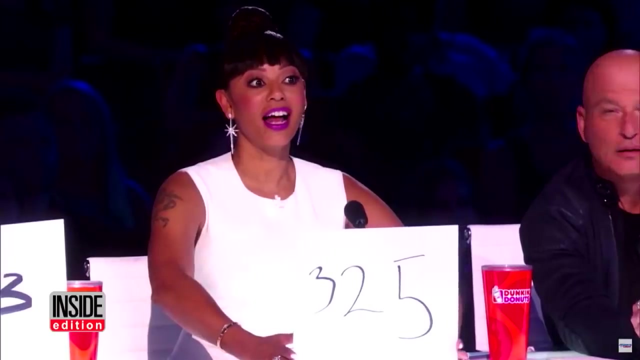 Mel B: 325.. Please peel off that sticker Without further ado. tell us all how many gumballs are in that jar. All right, 327.. Mel B was off by just two. But wait. the mentalists then stunned the audience playing this. 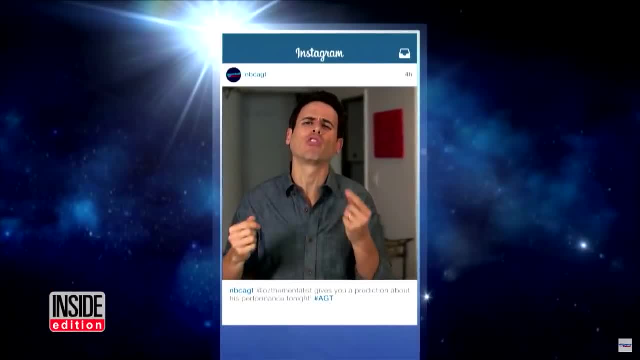 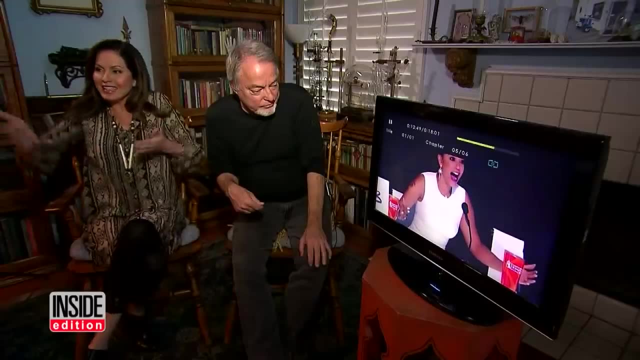 prerecorded message. What a big congratulations to Mel B, who was so close and off by just two gumballs. How did you do that? I know exactly how he did that: While Nick was peeling off the sticker, he was writing with his thumb on the back of the envelope. 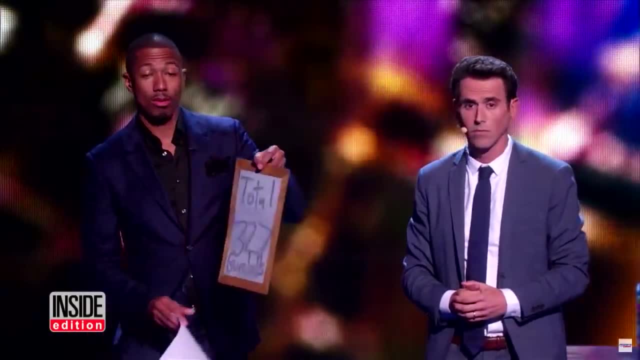 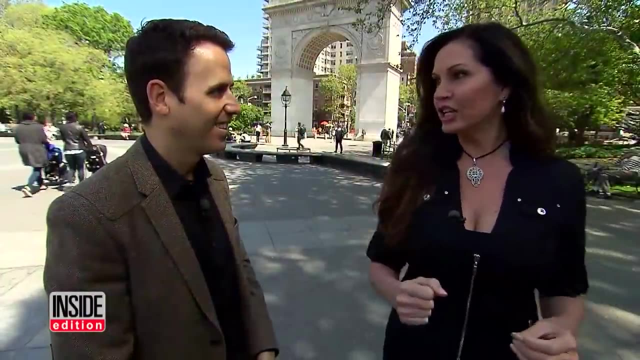 But inside the envelope is carbon paper, And so he wrote it after he saw her number. Do you hang out with magicians? No, I don't. I'm just very cynical. When Nick stood in front of you, were you writing the number? 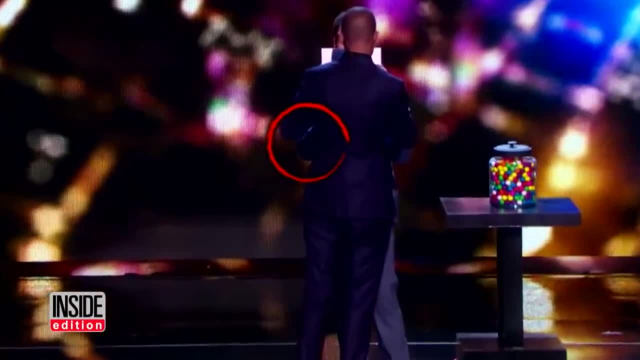 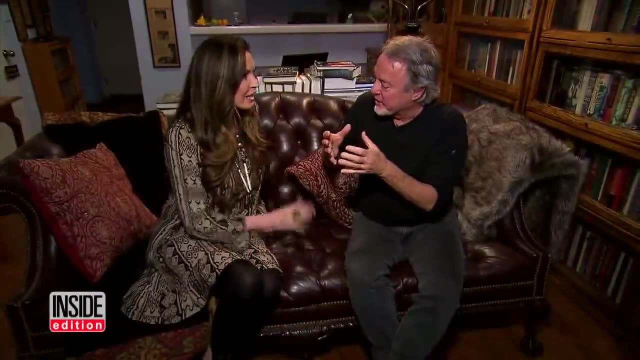 With your thumb on the back of the envelope as if it was carbon paper. You're not far off the trail. You're not dead on, but you're not far off the trail. So can anyone become a mentalist, Even me? 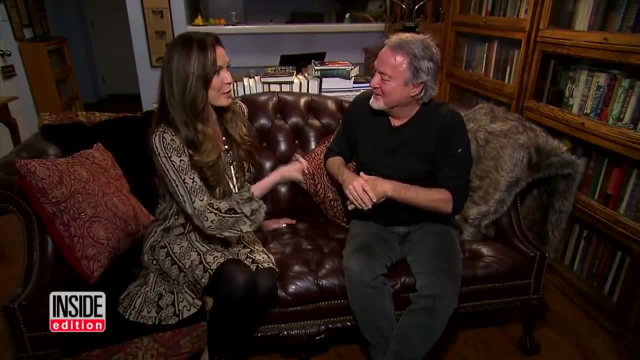 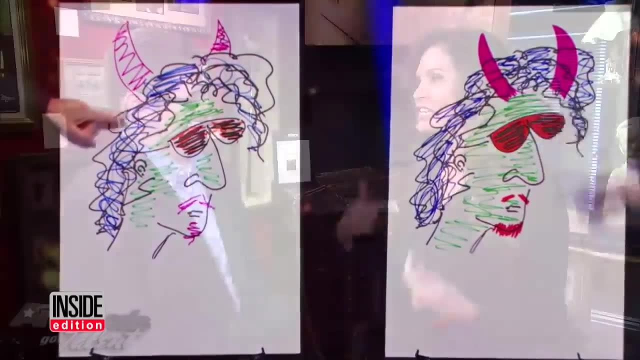 You could, Could I? Yes, I could learn how to be a mentalist. Yes, Eric Dittleman, a popular mentalist, was willing to train me. Whoa, Can you teach me a couple of things that I could maybe try to perform? 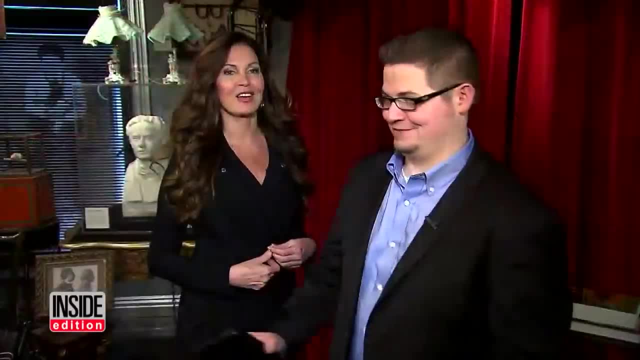 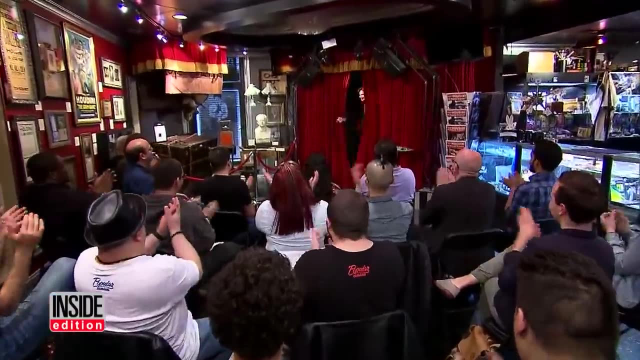 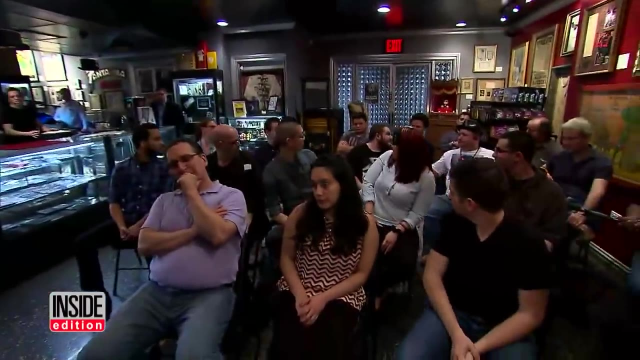 Yeah, we'll teach you a couple performances, some classics. It was showtime. Ladies and gentlemen, we're back. Ladies and gentlemen, mentalist Lisa Guerrero, I asked the audience to suggest a vacation location, which month to go and what should I do when I got there. 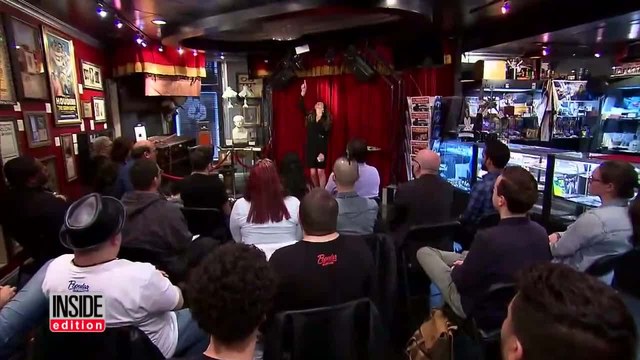 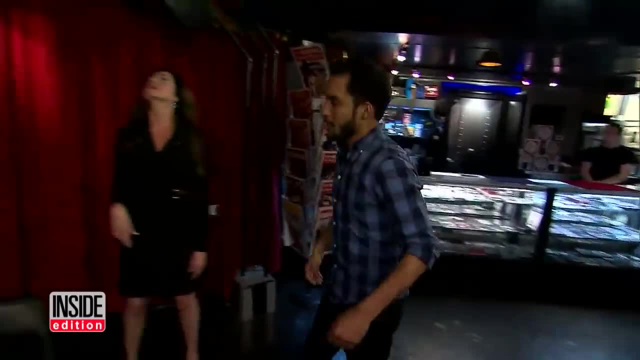 Disney World- July Ride Space Mountain. I told the audience that before the show I wrote down my predictions, put them in an envelope and hung it above me. Grab that and hand it to me And just get rid of the chair when you're done.